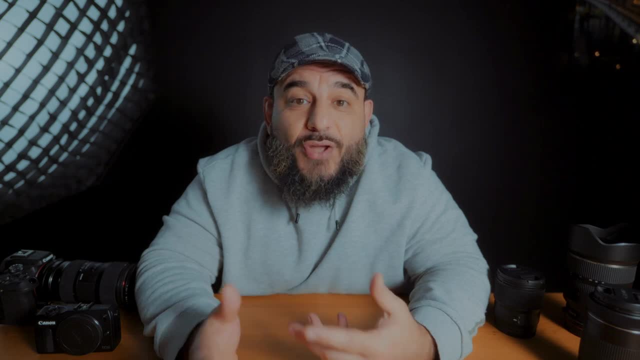 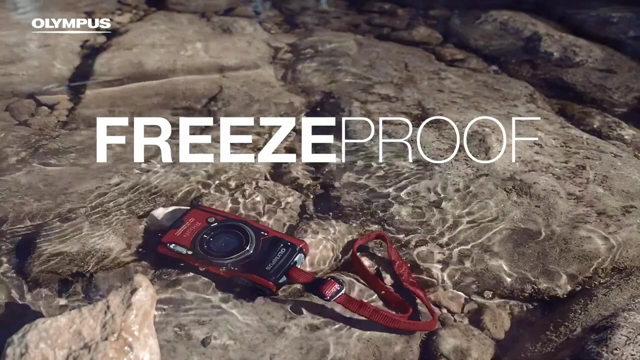 up to 220 pounds. So if you've been eating too many donuts and you accidentally sit down with this camera in your back pocket, you should be okay. And lastly, it's freeze-proof down to 14 degrees Fahrenheit. So basically, it's one of the 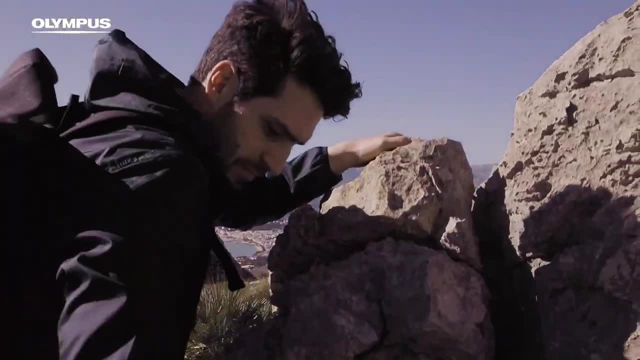 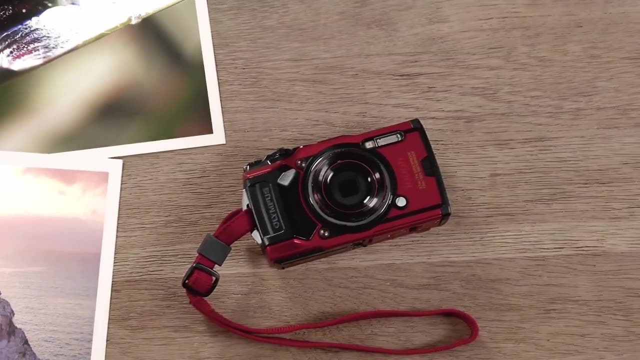 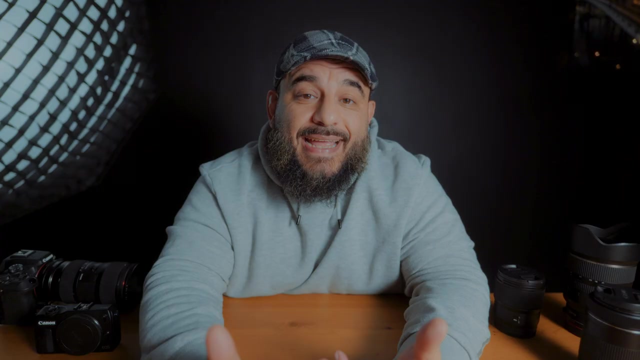 best cameras to have in your pocket if you plan on documenting an apocalyptic type of situation. Going back to the image quality, it has a 12 megapixel, 1 over 1.23 inch sensor and a fixed 25 to 100 millimeter equivalent F2 to F4.9 lens. It does have a built-in flash. 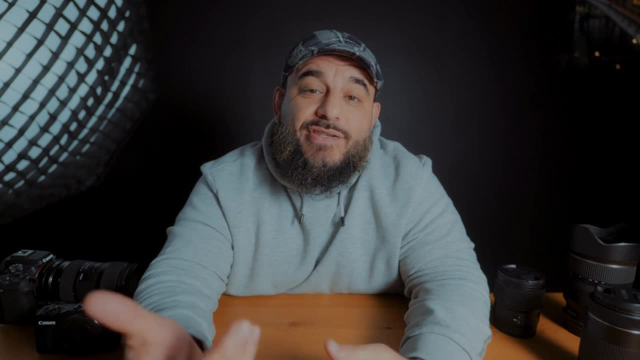 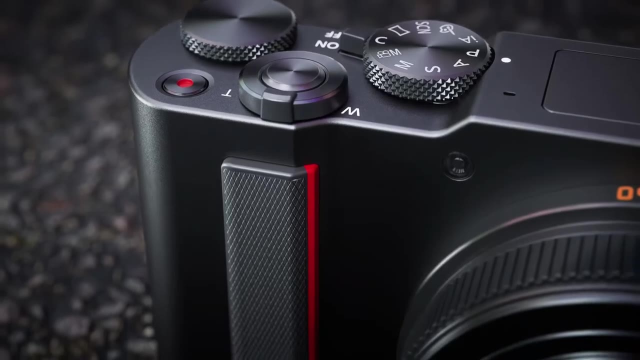 but unfortunately no EVF And there's no mic input, So you're stuck with the onboard mic when recording videos. Next we have the Lumix ZS200D, which is priced around 700 bucks and weighs 340 grams. It's. 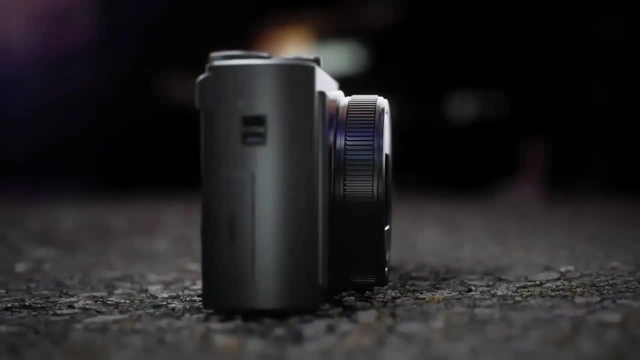 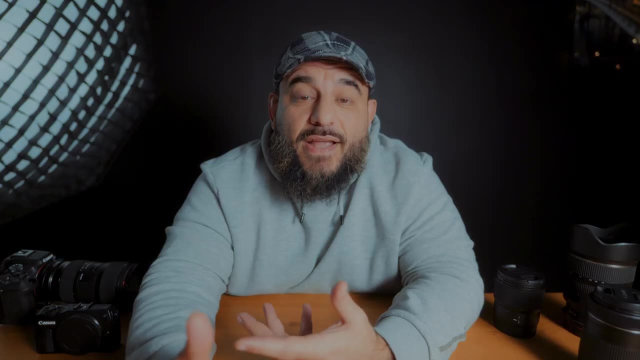 packing a 20 megapixel, 1 inch sensor and a 24 to 360 millimeter equivalent F3.3 to F6.4 lens. This provides you with 15 times optical zoom without losing any quality, making it an ideal compact camera for wildlife. 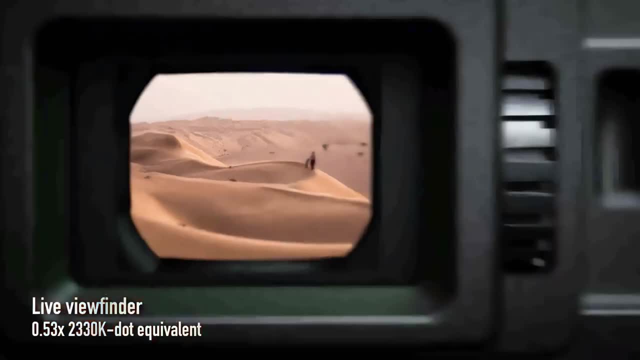 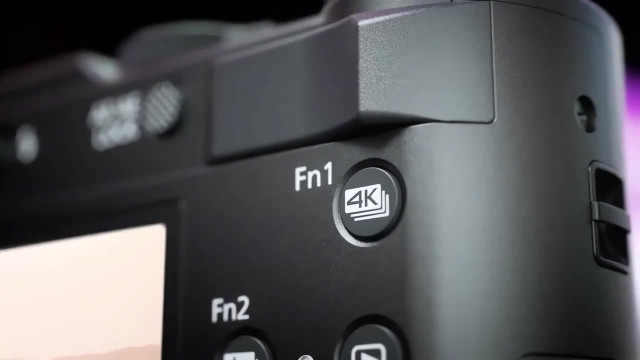 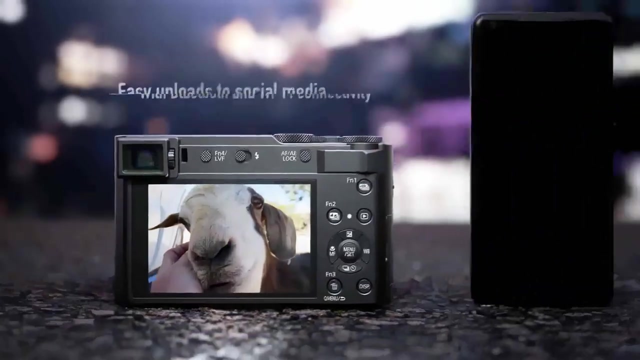 It also has a nice EVF and a pop up flash. You can shoot raw photos, 4K video up to 30 frames per second and 1080 up to 60 frames per second. It even has in-body image stabilization in video mode, which will reduce camera shake. 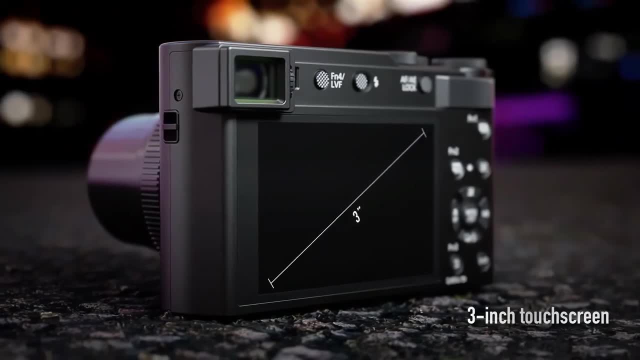 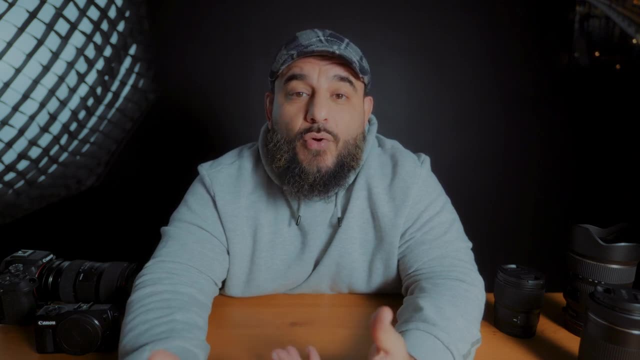 and micro jitters. Lumix also threw in a time-lapse feature, which can be a lot of fun. The cons are that you're stuck with the onboard mic because there's no mic input. Also, the aperture only opens up when recording videos. 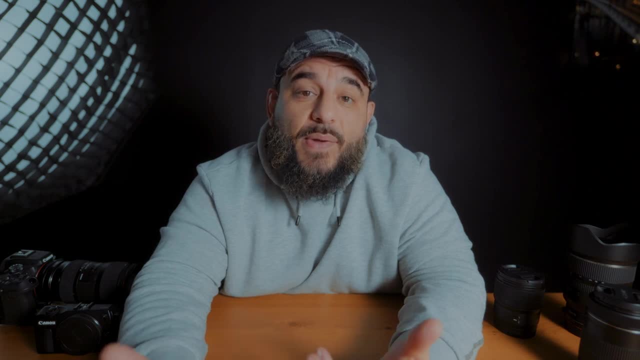 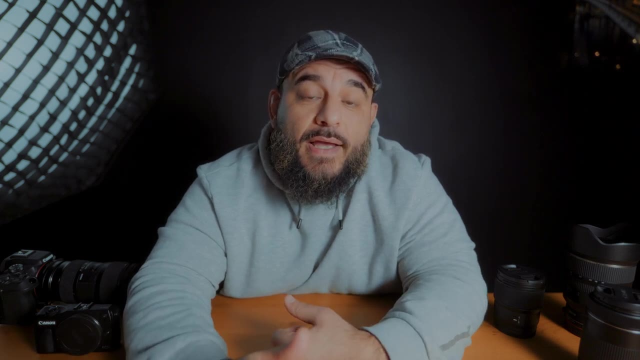 It opens up to F3.3 at its widest, so not the best for low light. That being said, this camera has the longest reach of any compact point and shoot that I'm aware of, So if that's your main focus- no pun intended- then this might be a good. 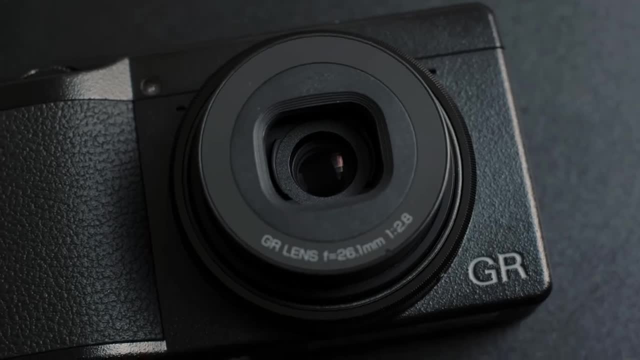 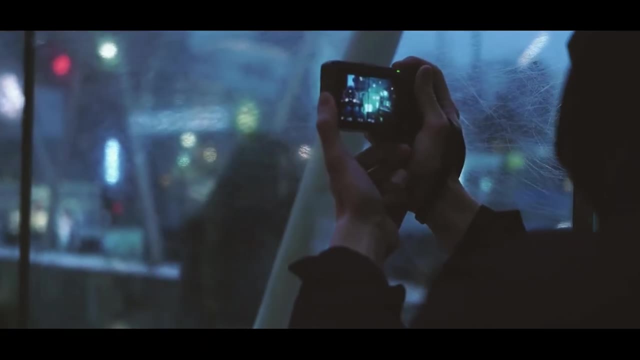 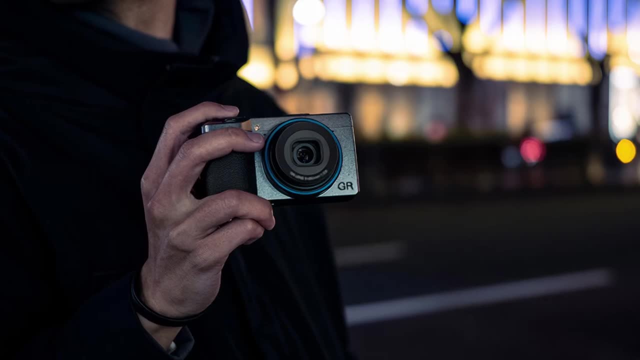 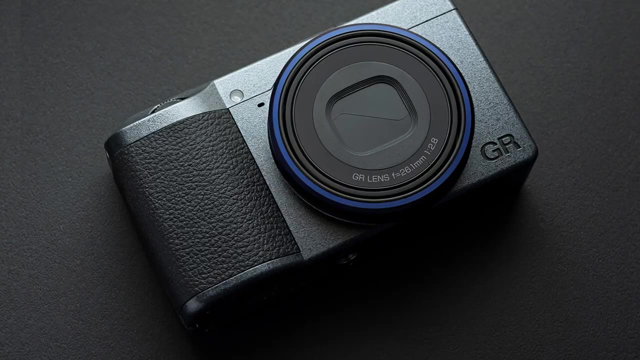 This camera is also available in this color scheme. It offers a 6 megapixel APSC sensor into this compact little body. The 40mm equivalent F2.8 lens gives you tack-sharp photos. This is a dream camera for many street photographers and it seems to have developed a cult-like. 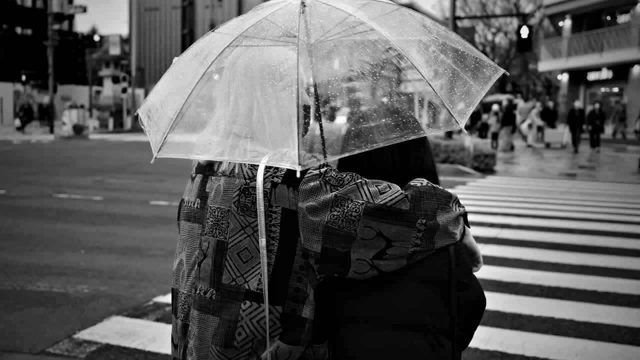 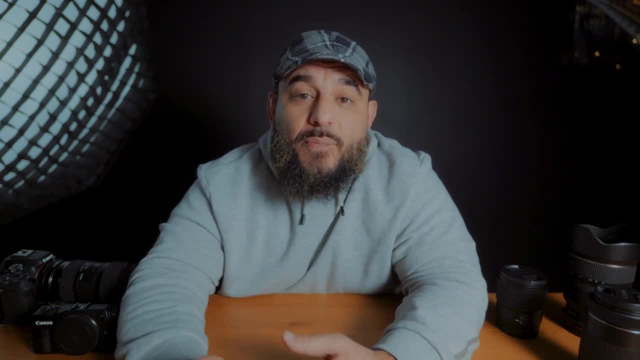 following, most likely due to its amazing image quality. The cons are that it doesn't have an EVF, The 3-inch screen doesn't rotate or tilt and the battery life could be a bit better. and it doesn't do that well at video. But 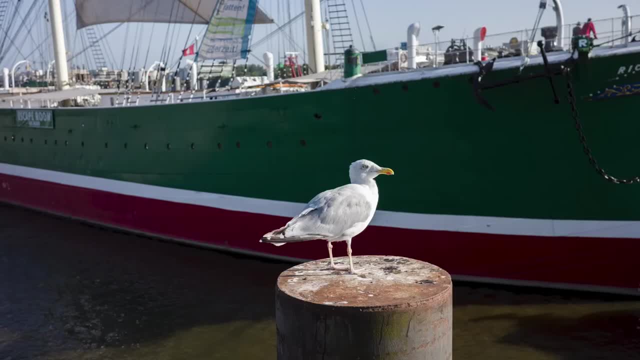 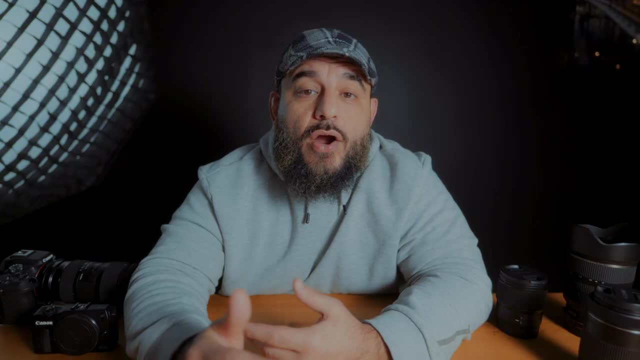 that's understandable, considering the target is 5KHZ target audience of this camera. If 40mm is too tight of a focal length for your style of street photography, you could opt for the original Ricoh GR3, which is a pretty similar camera, except that it has a. 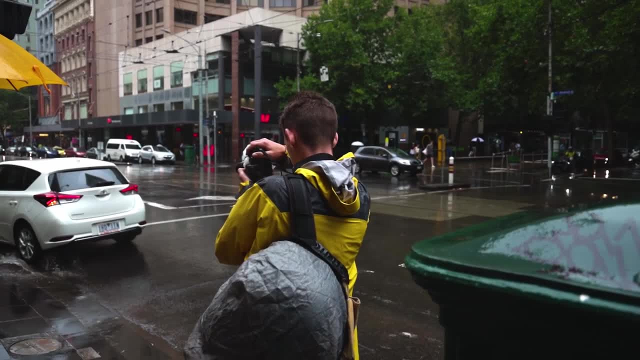 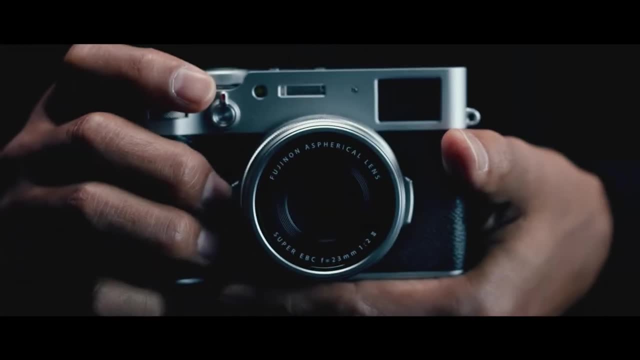 28mm equivalent lens. If you're a die hard street photographer, you could also go for the Fuji X100V, which has an even larger cult following than Ricoh cameras. It's not as compact, though. that's why I didn't include it in this list. 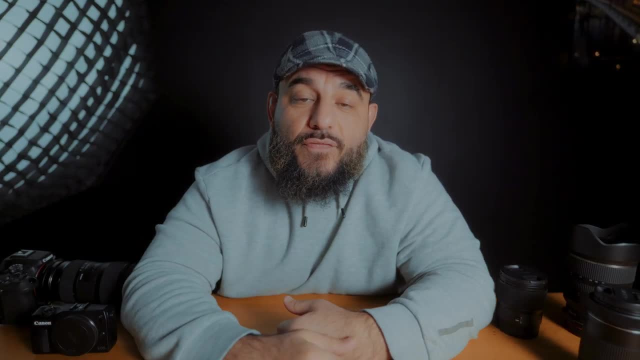 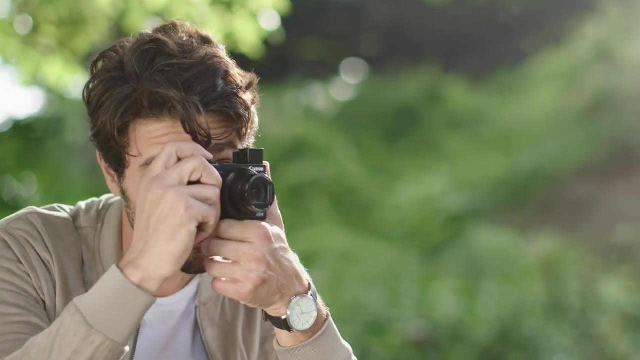 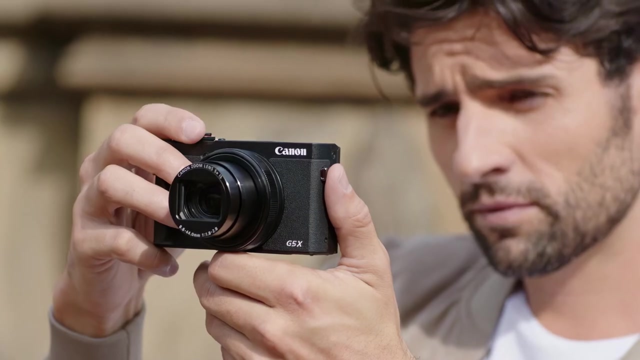 Nevertheless, I'll leave links below to all three of these street photography beasts. Next up, we have the Canon G5X Mark II. This camera comes in just under $900 bucks and weighs 340 grams. It packs a 20 megapixel, 1 inch sensor and a 24 to 120mm equivalent- f1.8 to f2.8- lens. 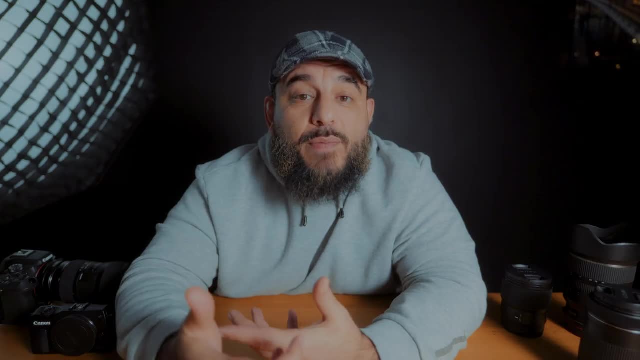 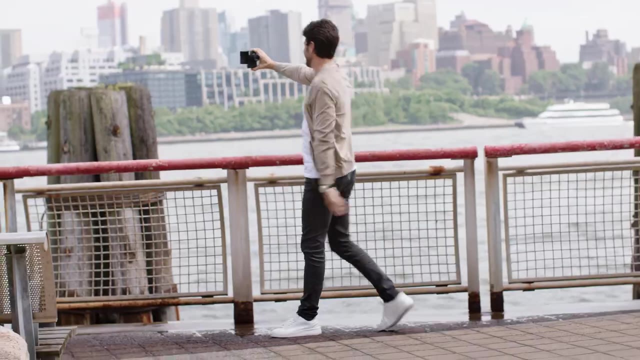 This gives you up to 5 times optical zoom while maintaining a pretty bright aperture throughout the whole focal range. The tilty screen allows for low angle shots, and it's ok for vlogging too. It also has a handy pop up EVF. Canon also threw in an internal ND for shooting in bright conditions. 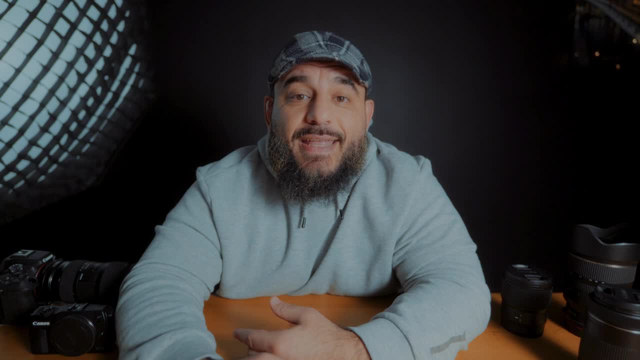 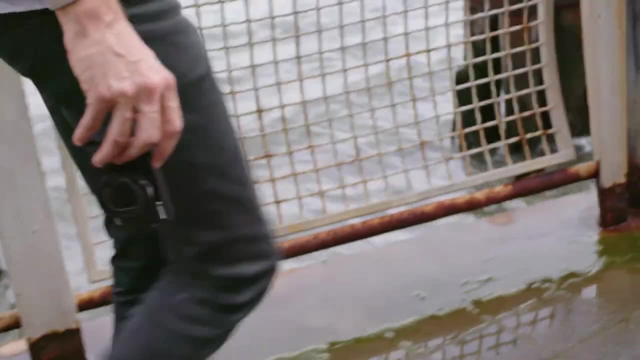 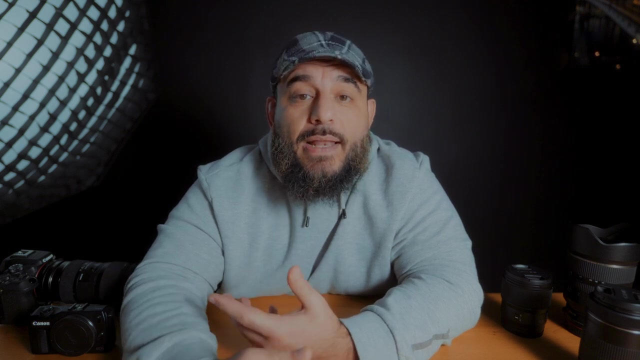 You could get 4K video up to 30 frames per second and 1080 up to 120 frames per second for some super slow mo footage. The ergonomics are also top notch, considering how small this camera is, and this is probably the easiest camera to use of all the cameras on my list. 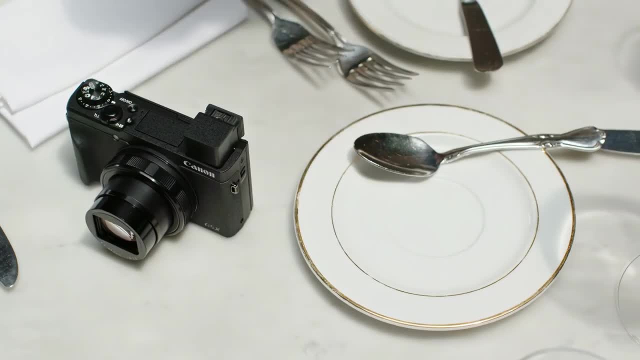 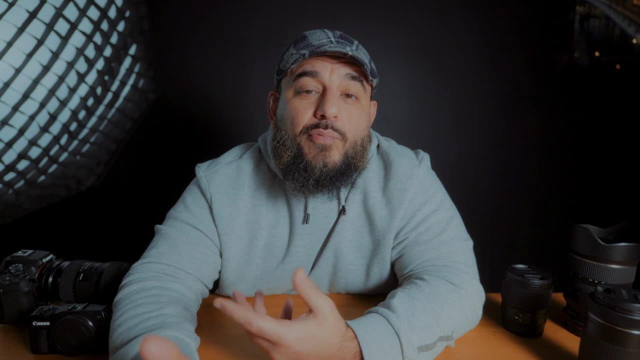 This is my number one pick If you're an enthusiast or casual shooter looking for a travel friendly compact camera to take photos of your friends and family. My only real gripe with the G5X Mark II is that it doesn't have a mic input and the 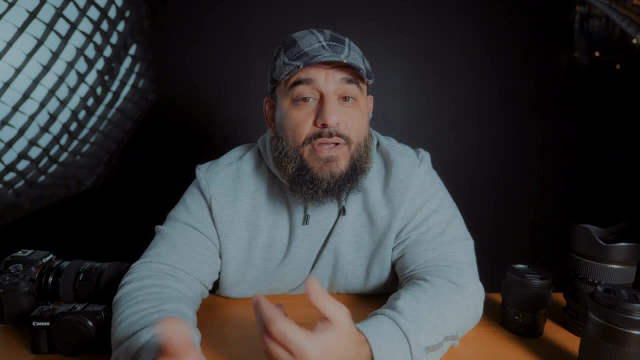 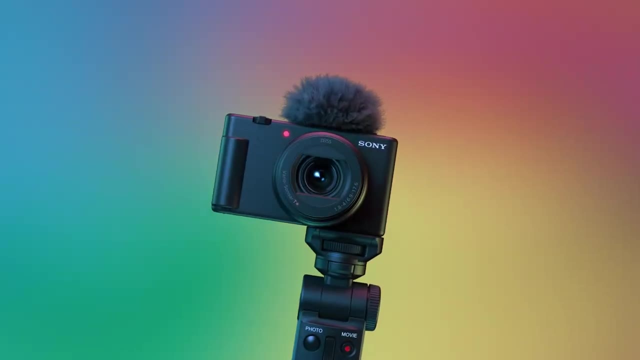 onboard mic isn't ideal. Other than that, it's a pretty good little camera. Coming in at number three, we have the Sony ZV-1 Mark II. This is the newest camera on our list, priced very fairly at about $900 bucks. 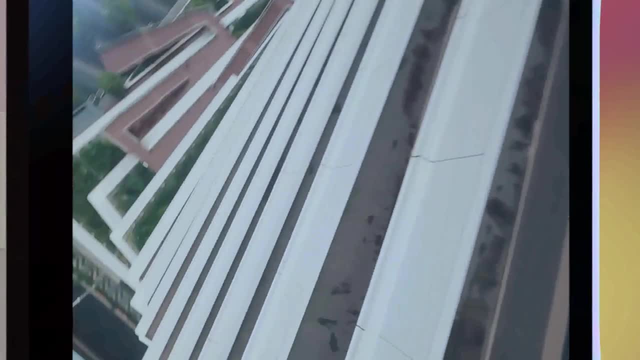 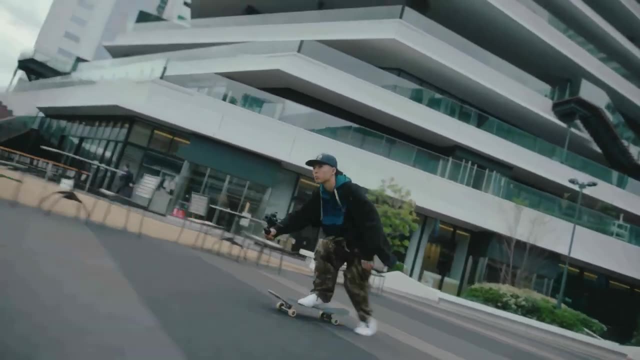 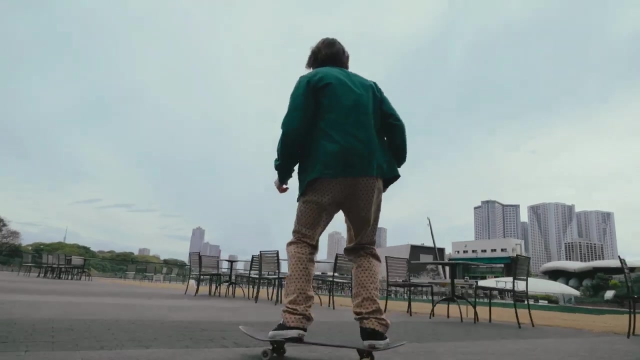 If your main focus is content creation, then this is the one for you. It also takes decent photos, but leans more towards the video side of things. It packs a 20 megapixel stacked 1 inch sensor and an 18 to 50mm equivalent- f1.8 to f4 lens. 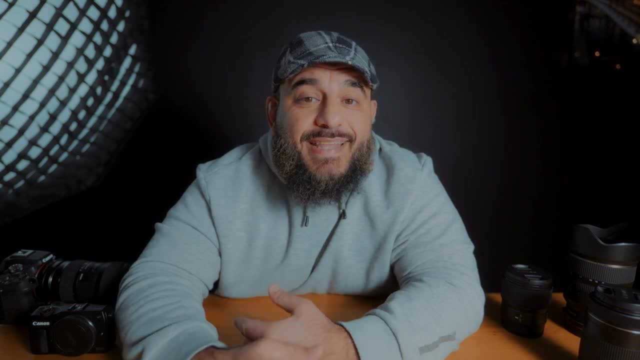 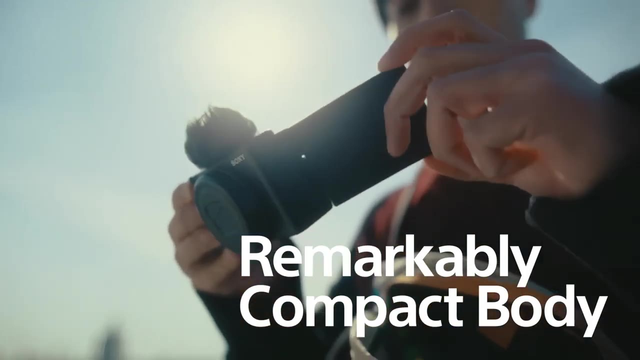 This gives you 2.7 times optical zoom, which isn't that much reach, but this is the widest lens of all the cameras on my list. The ZV-1 Mark II weighs 292 grams. It's a great camera to use for a lot of things. 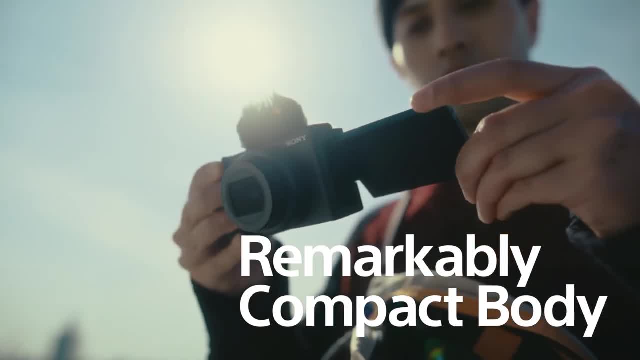 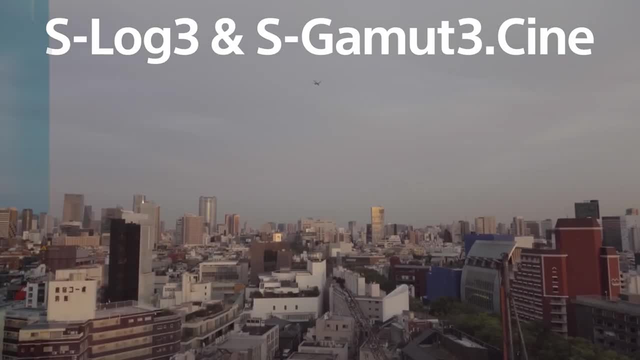 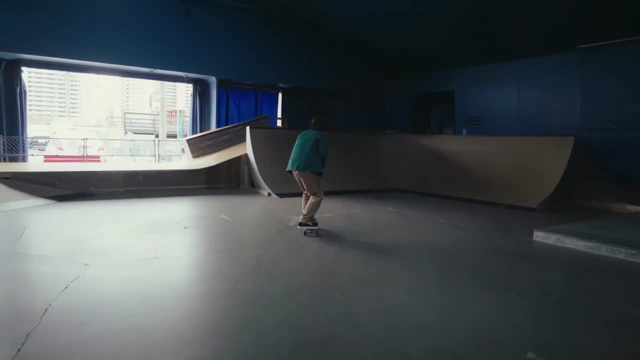 cameras that offers log recording. This is great for video shooters because it gives you better dynamic range and more flexibility when color grading. The auto focus in both video and stills is amongst the best out there, and it shoots video up to 120 frames per second. 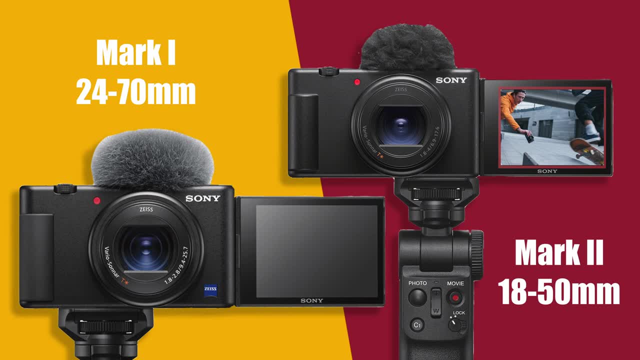 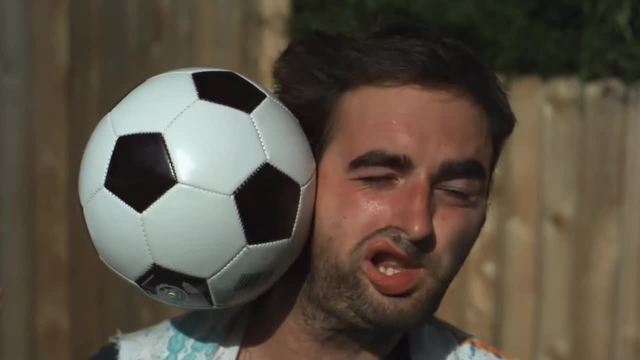 The original ZV-1 didn't have a lens this wide, but it did have up to 960 frames per second for super duper slow motion- slow motion which is unheard of in this price range. The main shortcoming of the ZV-1 series cameras is that they're lacking when it comes to. 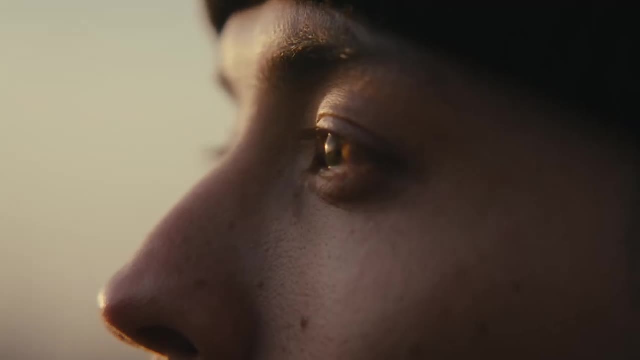 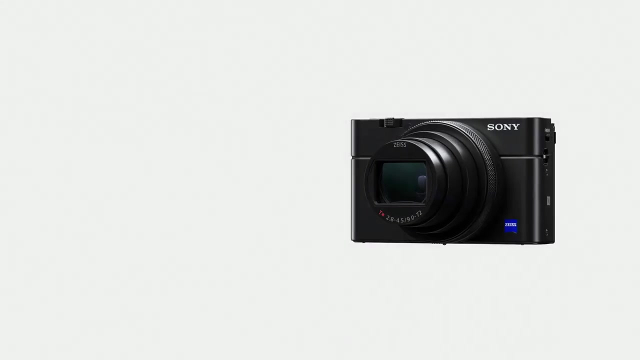 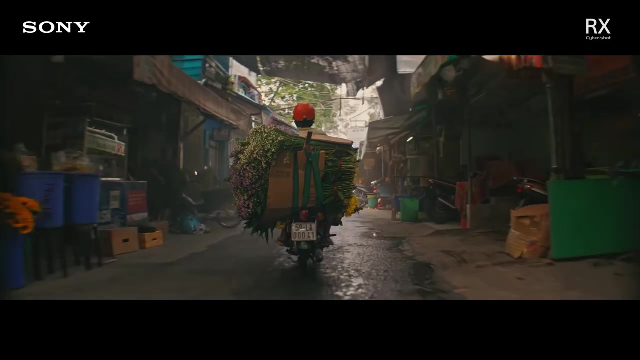 stills. It's not that you can't take good photos, but the lack of physical dials and buttons and no IBIS make photography a little more challenging. Coming in at number 2, we have the Sony RX100 VII. This is a very similar camera to the ZV-1 because it's great for content creation. 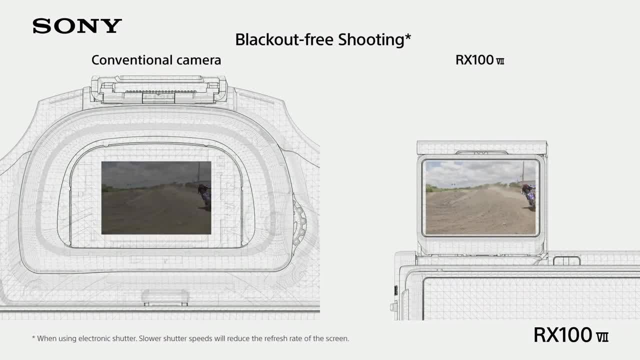 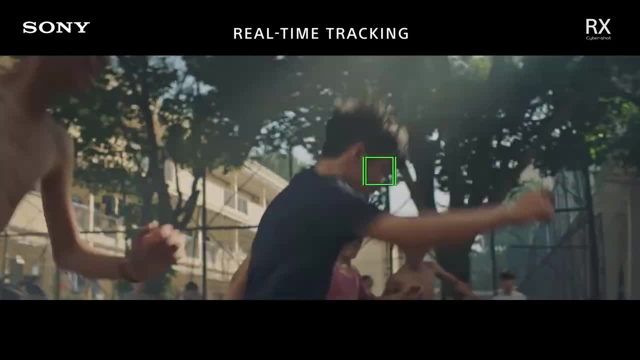 but it's also equally good at taking photos. If you're looking for an all-in-one compact content creation and photography camera, then this would be my number one pick. It's priced at about $1,100,, but it's worth the investment, in my opinion. 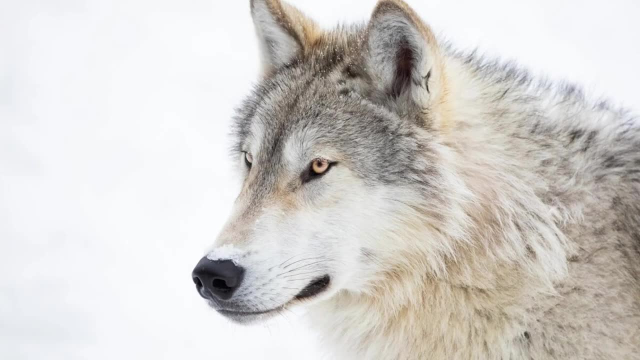 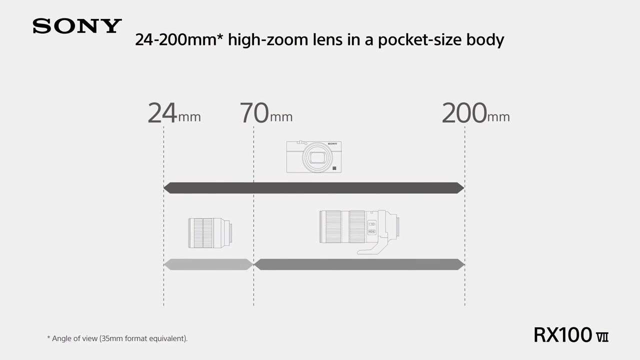 The 20-megapixel, 1-inch stacked sensor gives you amazing images. It has a 24- to 200-millimeter equivalent f2.8 to f4.5- lens. That gives you 8.3 times optical zoom and you get an additional 2 times digital zoom. 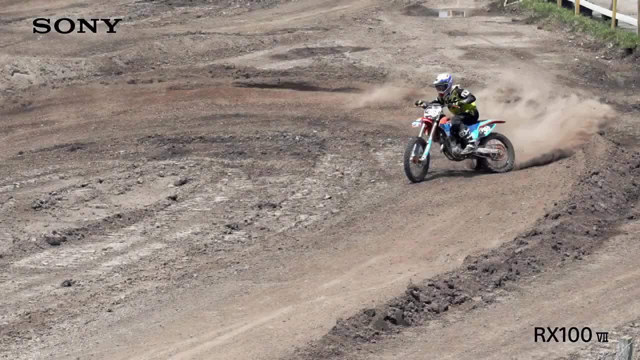 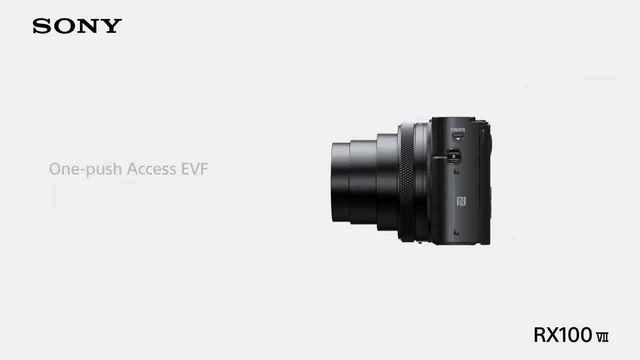 on top of that, Making the effective reach of this camera 400 millimeters. There's a 3-inch tilt-up screen, so it's good for low angle shots and decent for vlogging. It packs a nice pop-up EVF and even has a built-in flash. 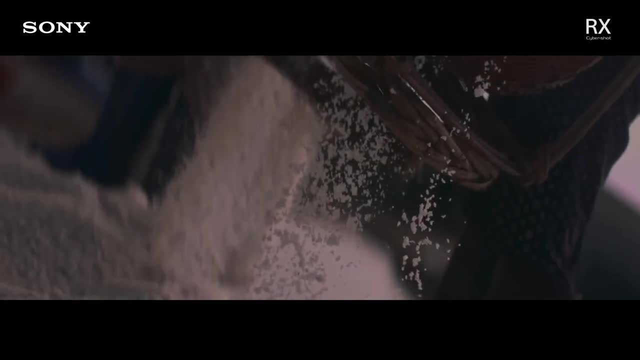 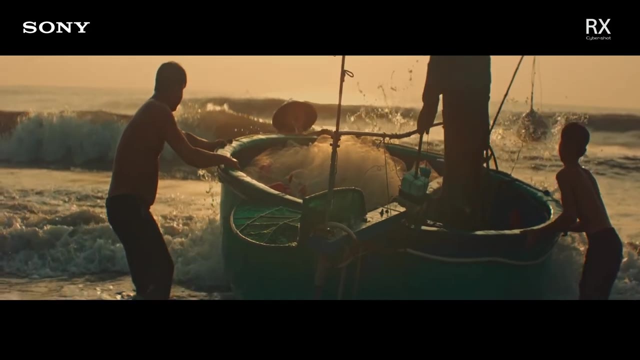 When it comes to video, it can shoot 4K up to 30 frames per second and 1080 up to 120 frames per second, And if you drop the resolution below 1080, you can even get 960 frames per second. 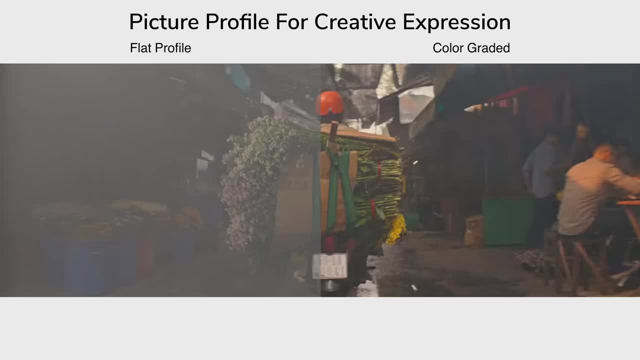 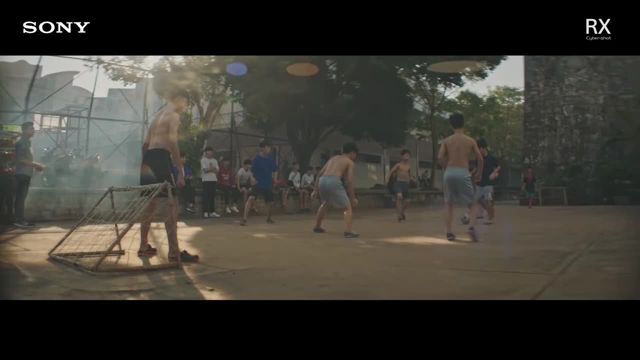 The autofocus is great in both stills. It has Sony's S-Log flat picture profile and an intervalometer for time-lapses. It has a mic input. it can shoot up to 20 stills per second with continuous autofocus and can do a whole lot more. 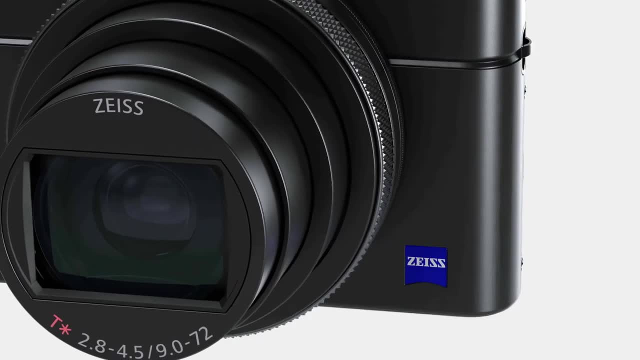 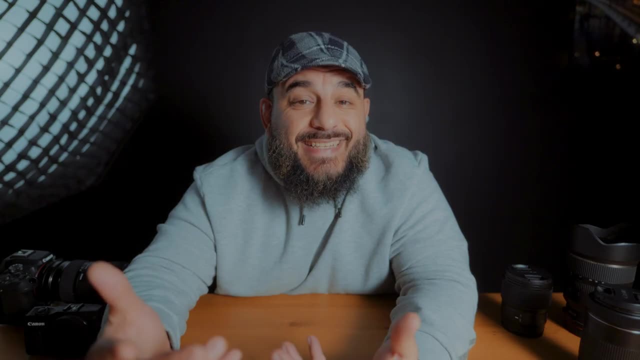 This is my number one pick for those looking for a compact fixed-lens camera that's equally good at photography and videography. And that brings us to my number one choice, which I think is going to be a little controversial, because some of you might not consider it to be a compact point-of-view camera. 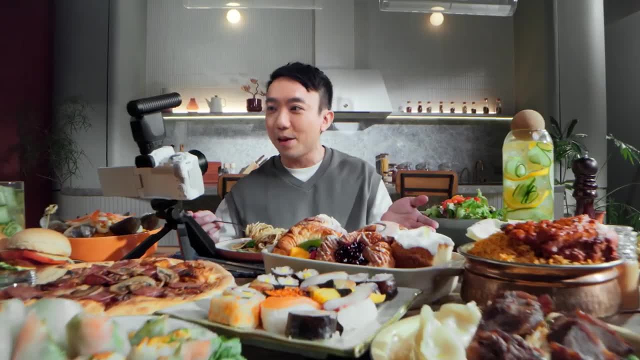 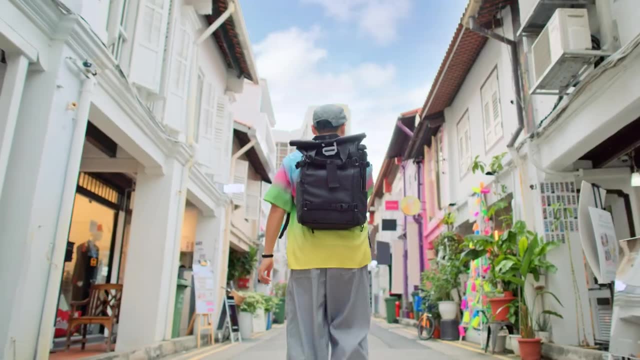 But it's not. It's going to be a compact point-of-shoot camera, But I kind of disagree. Here's the thing: Most of the cameras that I talked about weight around 300 grams or so. If you're willing to carry around an additional 100 grams, then you could get an interchangeable. 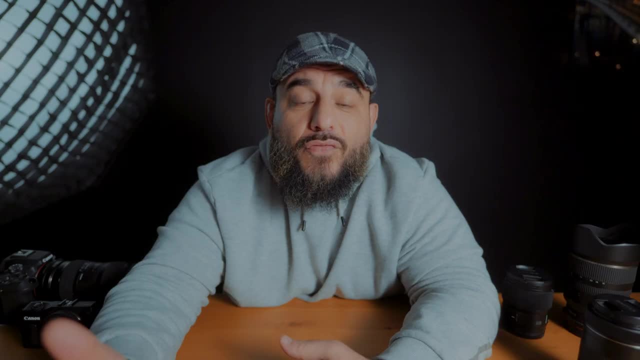 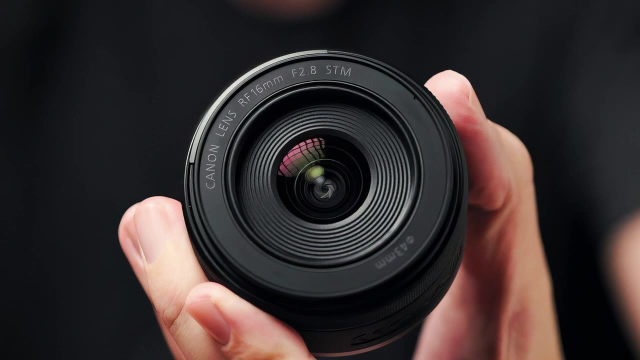 lens camera which would allow you to do everything from street photography to wildlife just by swapping out a lens. Take, for example, the Canon RF 16mm f2.8 pancake lens. If you slap that onto the Canon R50, you'd still be able to force the whole setup around.